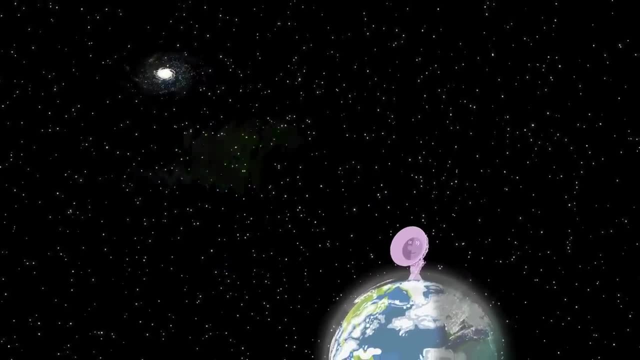 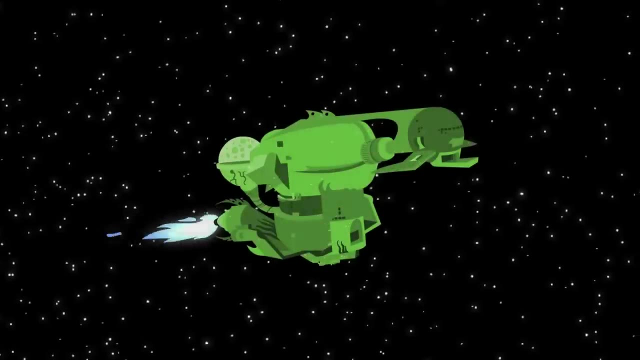 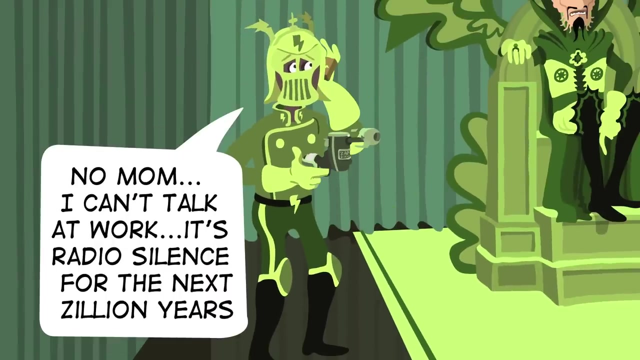 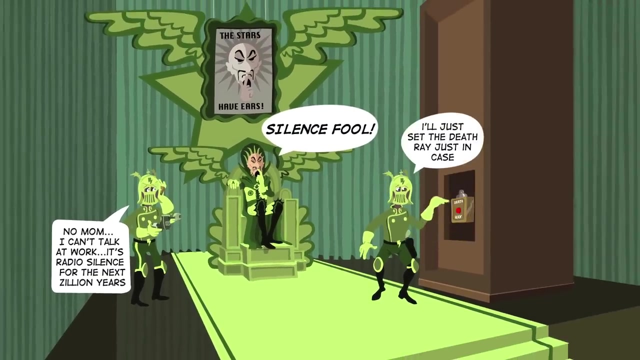 of any of it. Why? Well, there are numerous possible answers, some of them quite dark. Maybe a single super-intelligent civilization has indeed taken over the galaxy And has imposed strict radio silence because it's paranoid of any potential competitors. It's just sitting there ready to obliterate anything that becomes a threat. 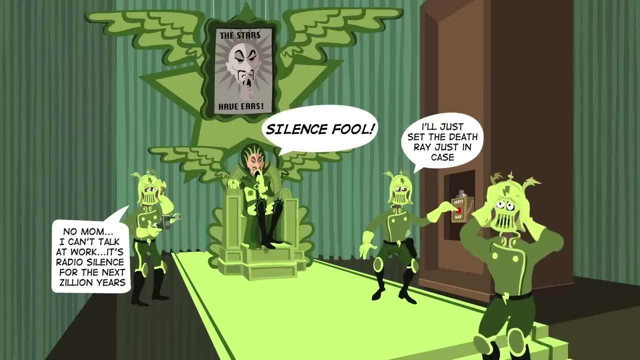 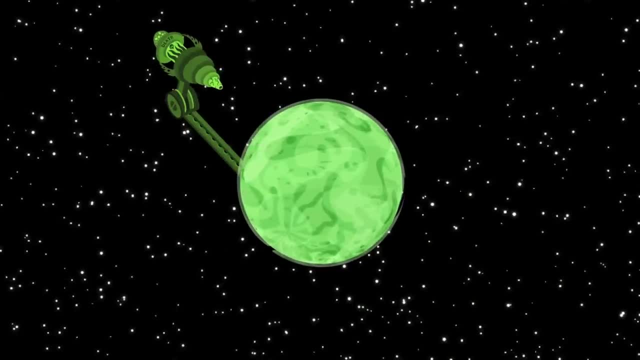 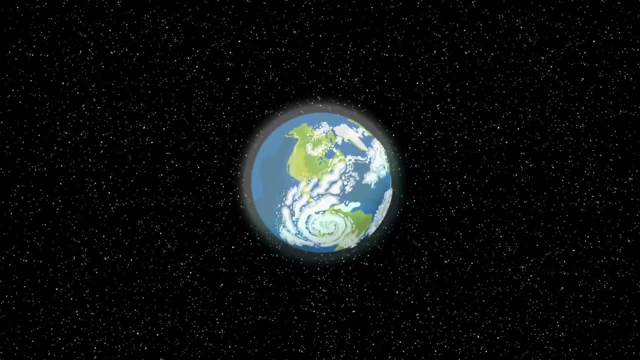 Or maybe they're not that intelligent, Or perhaps the evolution of an intelligence capable of creating sophisticated technology is far rarer than we've assumed. After all, it's only happened once on Earth in four billion years. Maybe even that was incredibly rare. 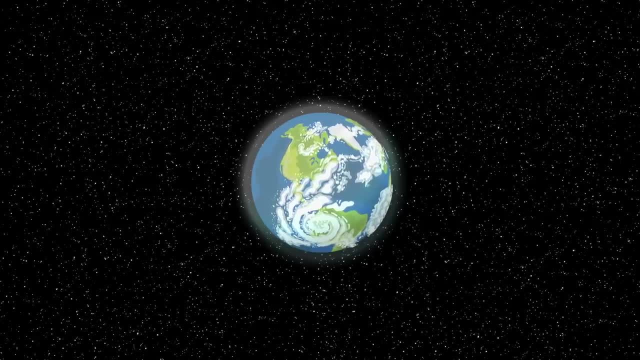 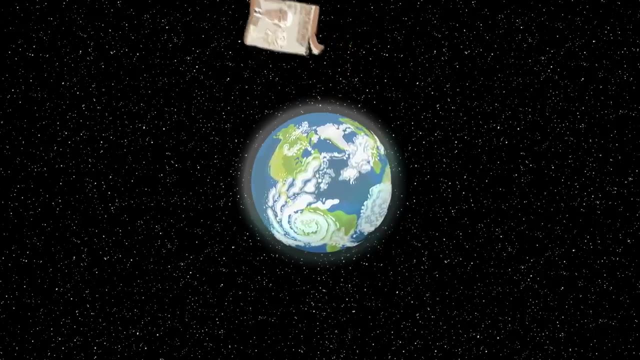 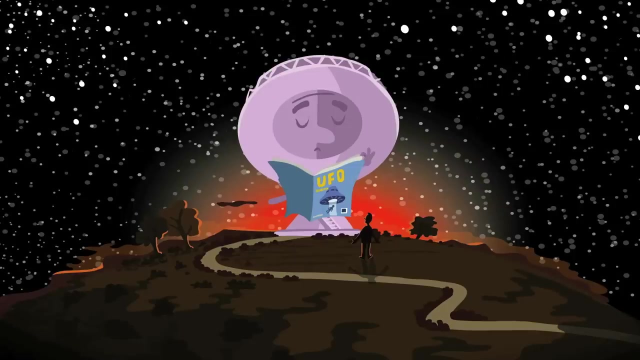 Maybe we are the first such civilization in our galaxy, Or perhaps civilization carries with it the seeds of its own destruction through the inability to control the technologies it creates. But there are numerous more hopeful answers. I mean, for a start, we're not looking that hard and we're spending a pitiful amount of money on it. 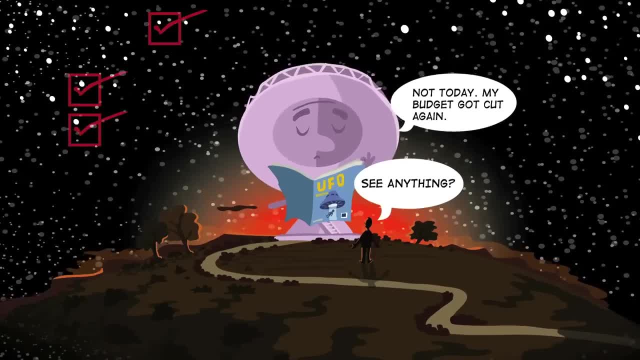 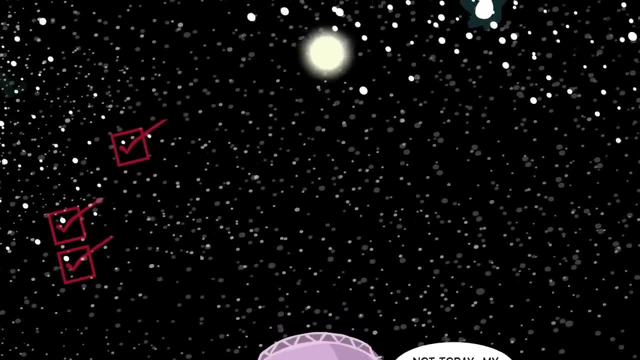 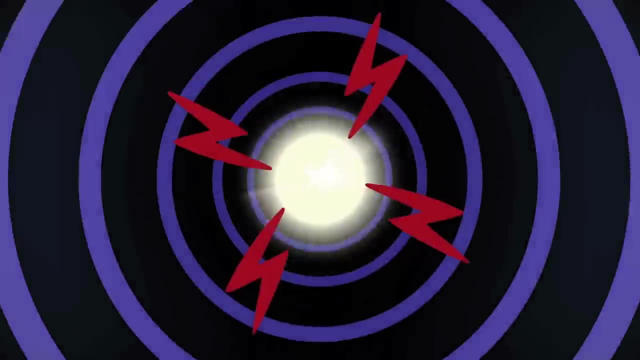 Only a tiny fraction of the stars in our galaxy have really been looked at closely for signs of interesting signals, And perhaps we're not looking the right way. Maybe, as civilizations develop, they quickly discover communication technologies far more sophisticated and useful than electromagnetic waves. 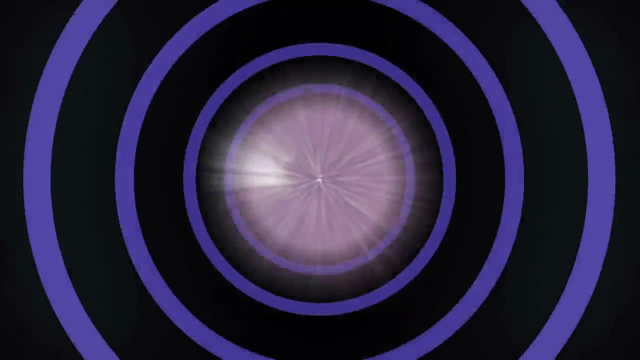 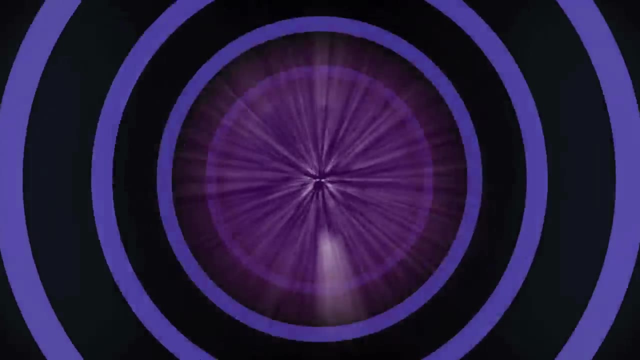 Maybe all the action takes place inside the mysterious recently-discovered dark matter or dark energy that appear to account for most of the universe's mass. Or maybe we're looking at the wrong scale. Perhaps intelligent civilizations come to realize that life on Earth is just a matter of time. 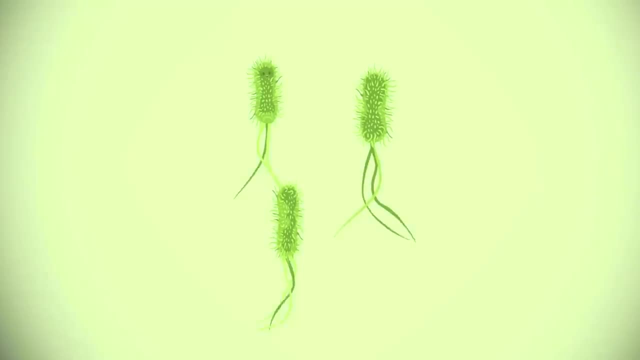 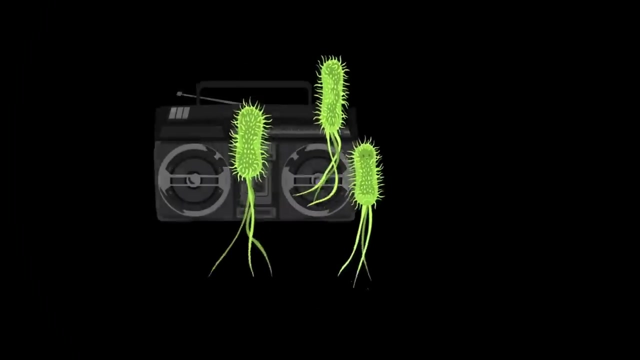 Or maybe we're looking at the wrong scale, That life is ultimately just complex patterns of information interacting with each other in a beautiful way, And that that can happen more efficiently at a small scale. So just as on Earth, clunky stereo systems have shrunk to beautiful tiny iPods. 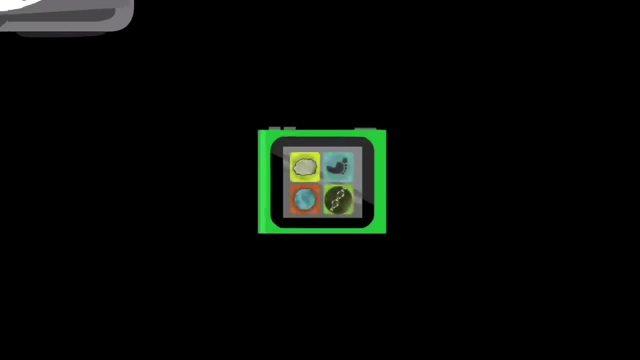 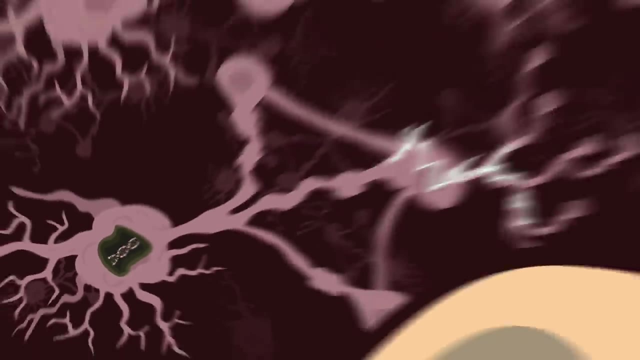 maybe intelligent life itself, in order to reduce its footprint on the environment, has turned itself microscopic, So the solar system might be teeming with aliens and we're just not noticing them. Maybe the very ideas in our heads are a form of alien life.